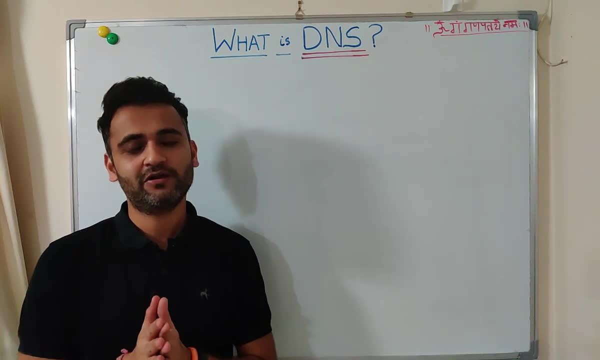 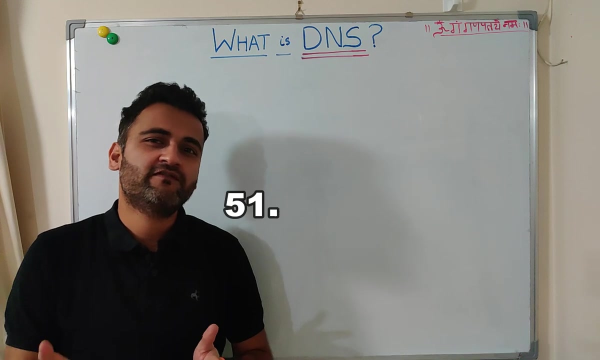 friend and he casually asked me which is your favorite tourist location in United Kingdom? And I replied that yes, I do have a location. And he asked: okay, so which location do you like the most? And I said it's 51.505 degree north and 0.0754 degree west. That's the location I like to visit. 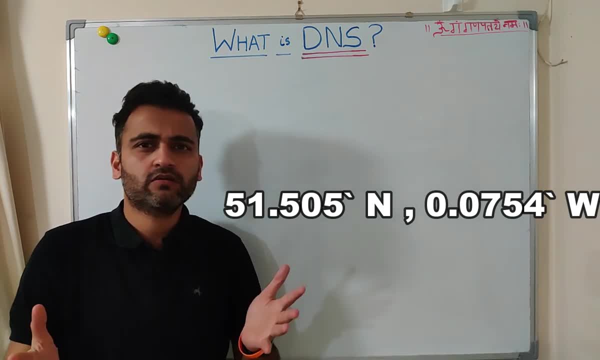 time and again. He was shocked. He said: okay, but what is it? I said this is the location which I like to visit again and again. But my friend said: what is the location? I said I told you. 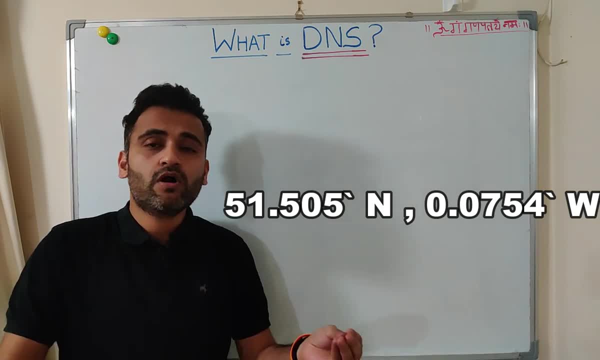 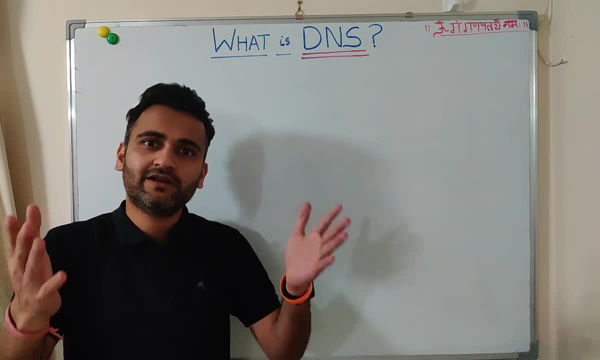 this is the location. But what does that mean? I said this is the coordinates for my favorite location. Now he was getting irritated So I jokingly said: okay, I was kidding, And the location which I was talking about is Tower Bridge in London. 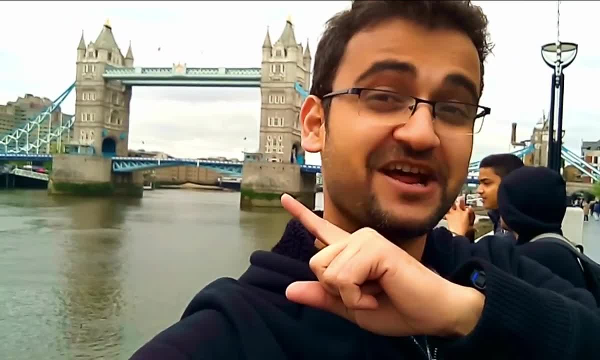 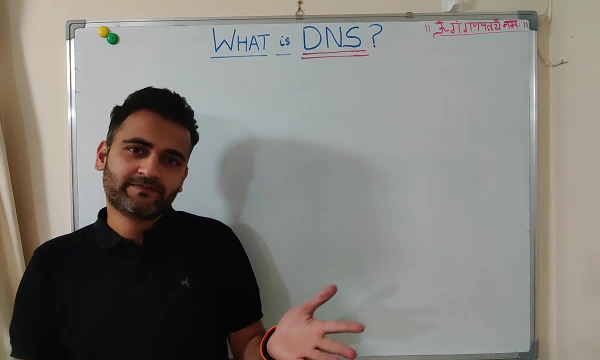 I'm back at Tower Bridge. Then he asked me: why didn't you tell that in the beginning? I said I thought you would understand the coordinates. Now take that example and just simply understand how many computers are today. They are connected with each other. 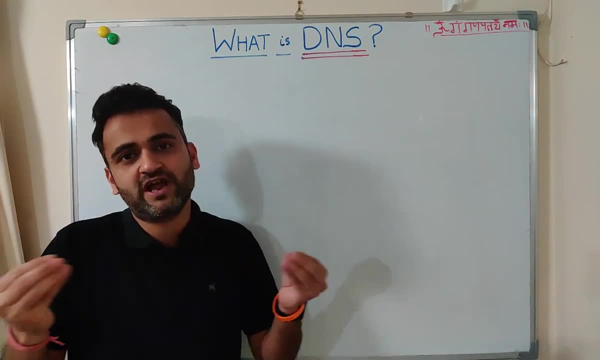 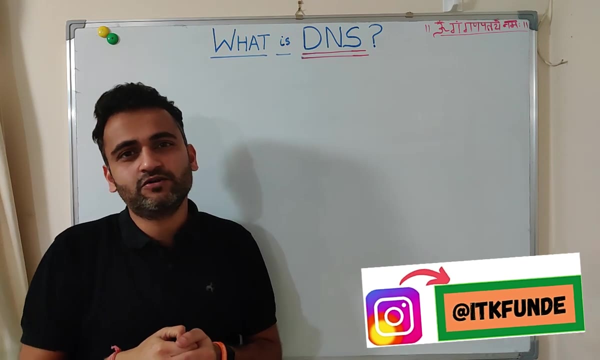 You anyways know that every computer is actually identified with its IP address. But if you have to remember the IP address of all the networking devices you interact with, all the computers, all the servers, it would be a Herculean task. It is impossible for a human, Because we are not. 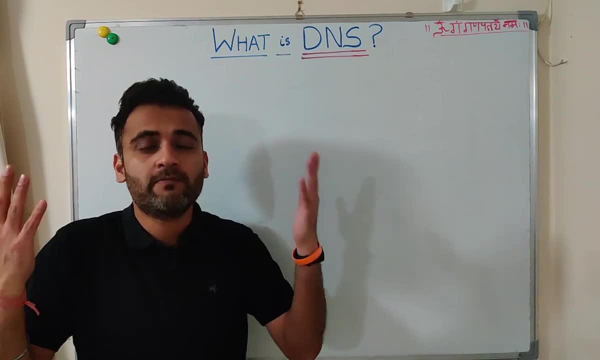 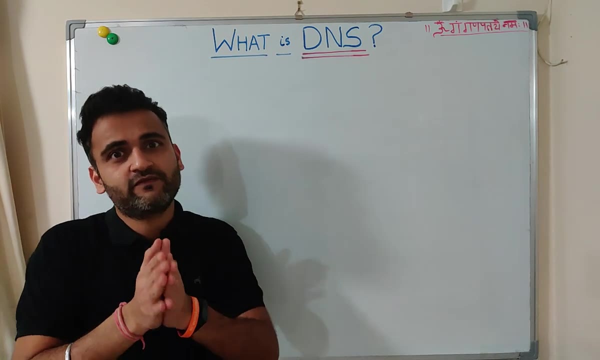 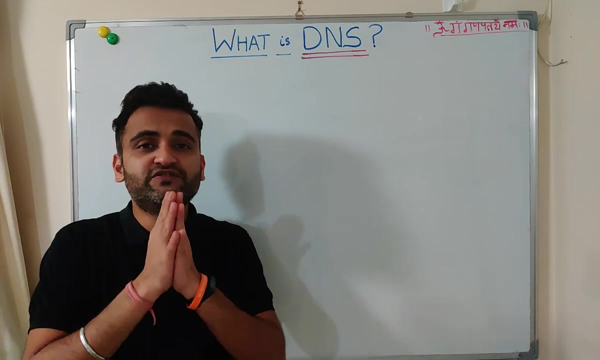 robots. We are humans, And humans generally are not very good at remembering numbers, And same is the case with remembering IP address. So in that case, the rescuer for us is the domain name. DNS is the facility, is a TCP IP facility which provides us with a unique name to one particular. 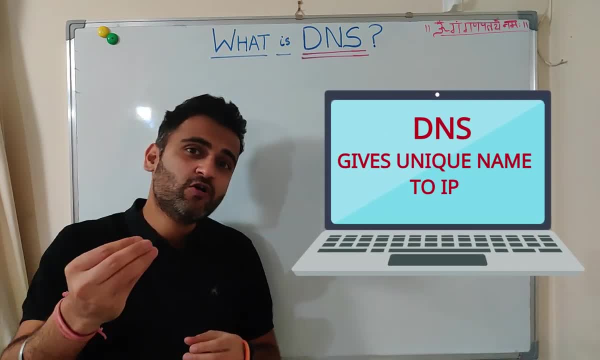 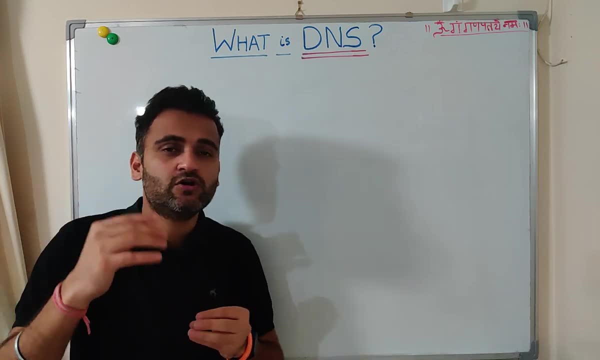 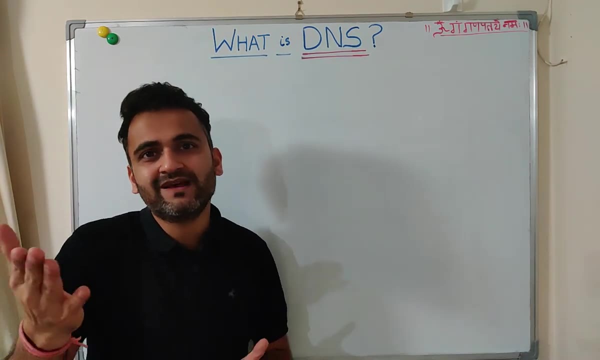 server or one particular device over the network. So instead of remembering the IP addresses of, you know, of all the websites which you access- for example googlecom, amazoncom- all these are- actually eventually end up being an IP address on the network. Suppose you want to buy something on. 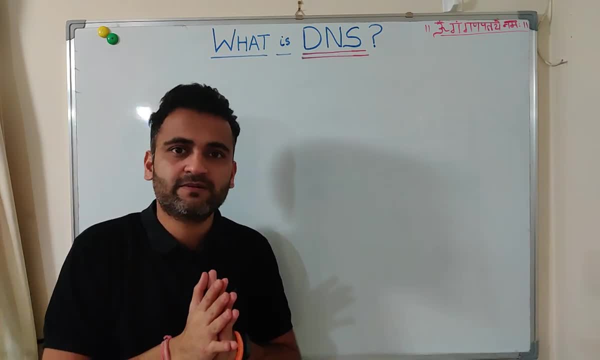 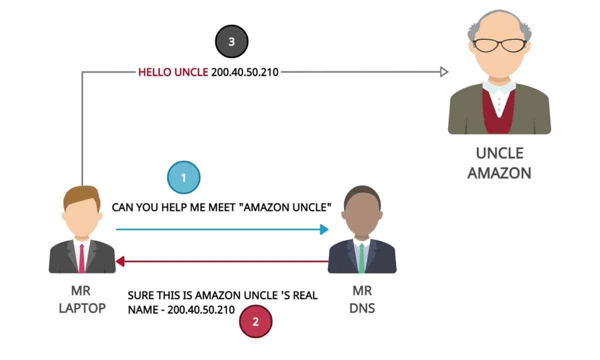 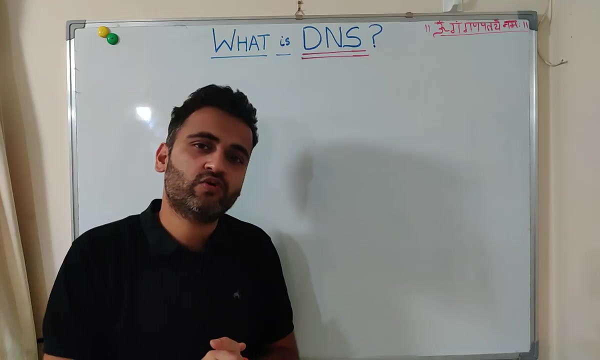 Amazon. You need to know the IP address of that particular server because Amazon has so many servers across the globe. So you you simply write wwwamazoncom and the DNS server will get the IP address- you know which- which will be used to connect to Amazon servers. So now with that basic, 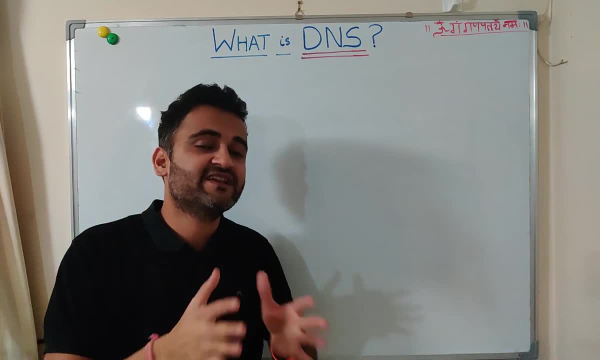 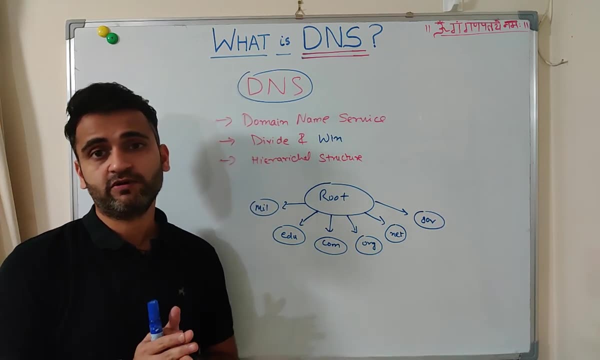 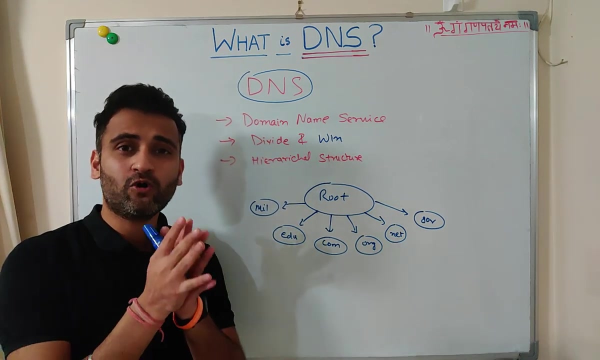 understanding. let's understand in more detail what is a DNS and how exactly it works. So you must be wondering how DNS manages so many names because there are so many servers in this. you know, in this world of internet, The DNS uses a very simple policy of divide and win. it divides all these namespaces, all these. 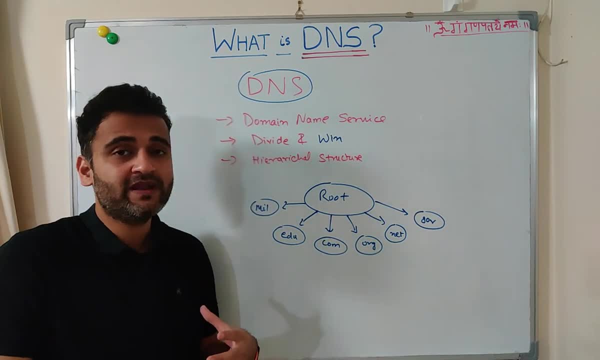 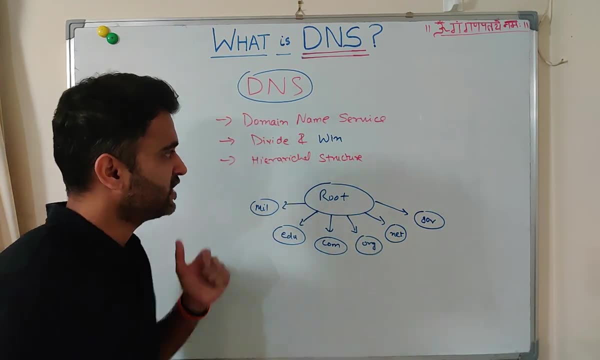 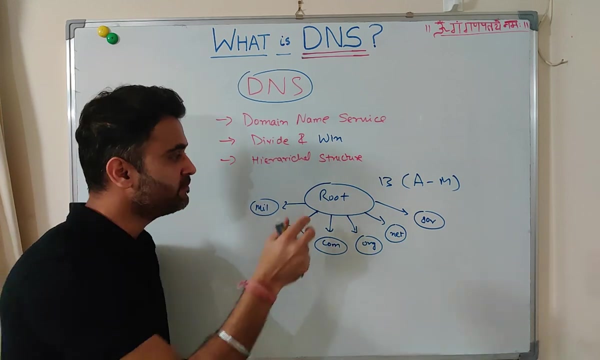 unique names in different domains. we will understand what is a domain now. So, basically, you have one particular root domain And there are different around 13 root domains across the globe And the names are from A to M, So every domain name actually belongs to this root. this root is the. 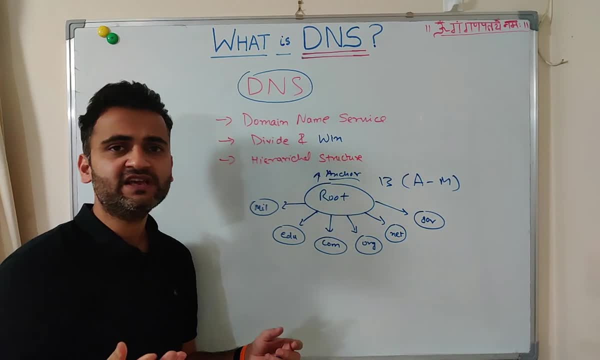 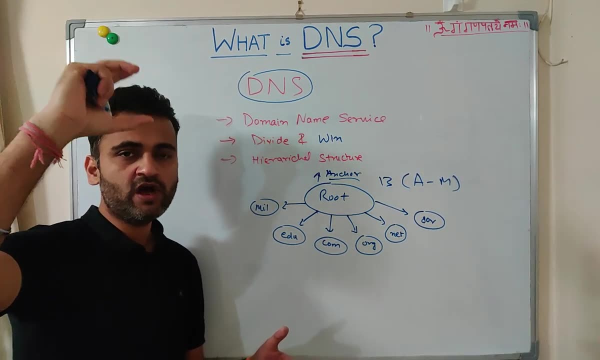 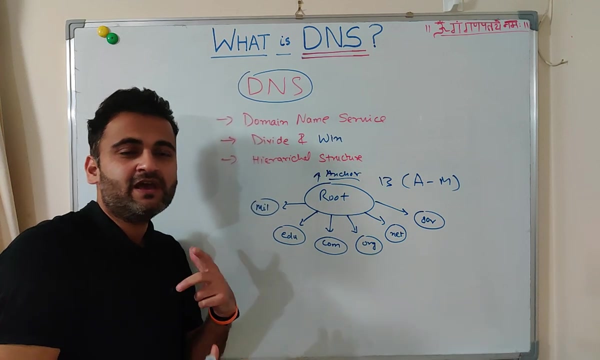 anchor point And any, any name which you see actually belongs to this particular root. So the root is kind of the parent, parent node And under that you have the hierarchy, because obviously domain name follows an hierarchical structure which you see maybe in your Windows folder. you have a folder, then you have a sub folder. 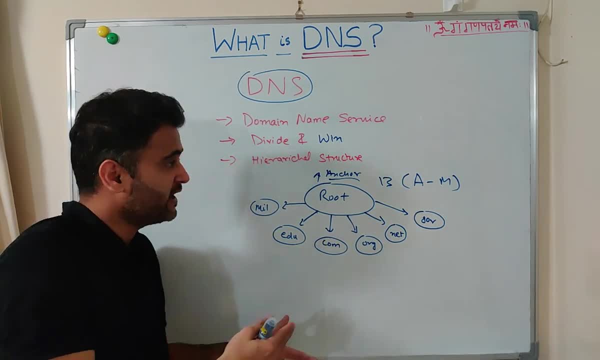 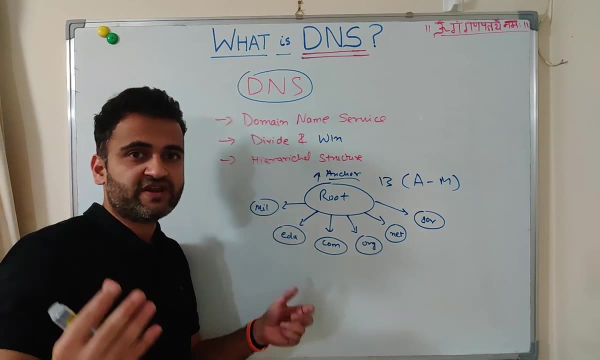 then you have multiple folders under that sub folder. In a similar way, DNS also use that hierarchical nature. So there is a root domain- there are 13 different root domains already established across the globe- And then you have a sub folder, then you have multiple sub folders. 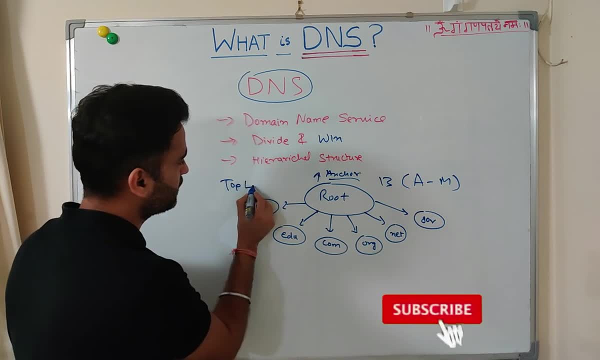 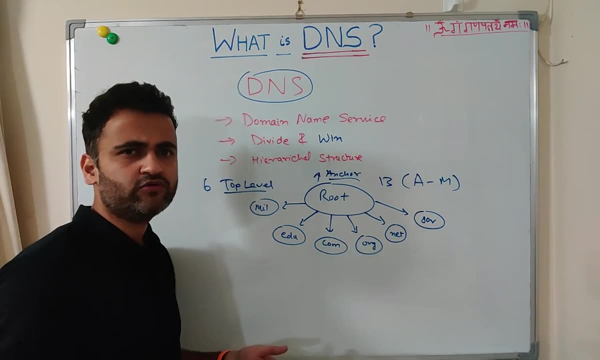 And under that you have top level domains. So there are quite well defined top level six, six top level domains. Now there are some new ones also which have been introduced. I think there are seven new top level domains which have been introduced, But these are the main six top level domains. 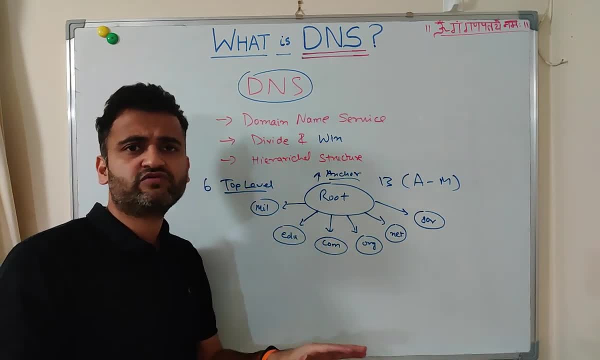 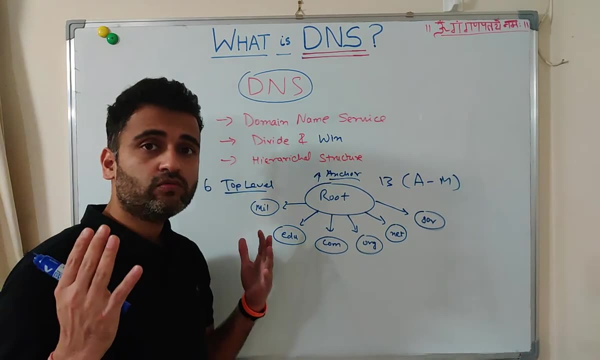 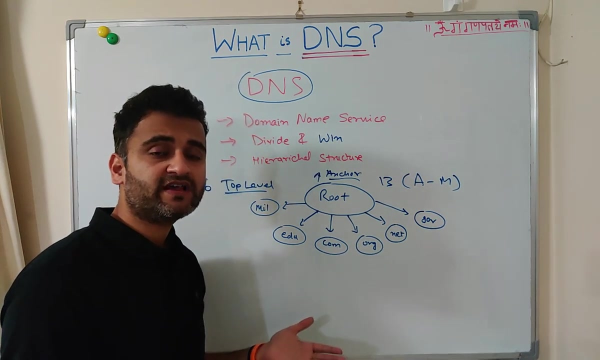 which you might have seen. in pretty much any website which you try to enter, any address you try to enter it- it eventually will end up with any of these top level domains. So just quickly, I'm just what these top level domains are used for. so dot mill is used by military setup and military. 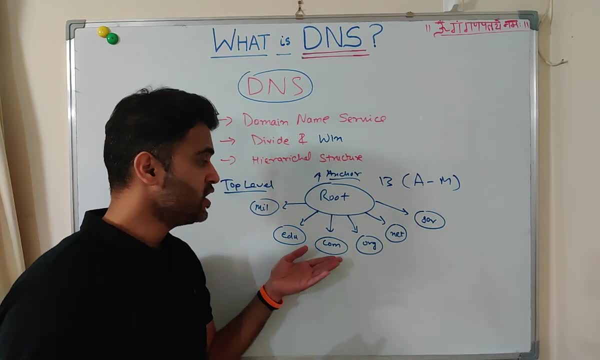 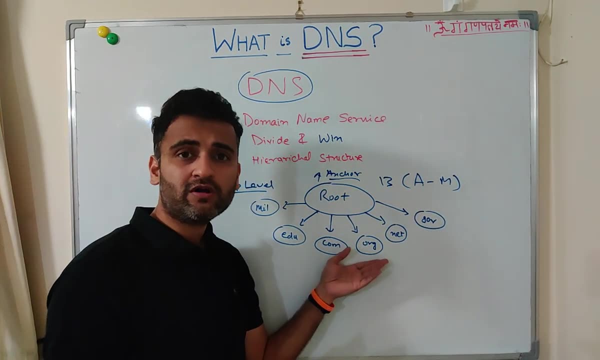 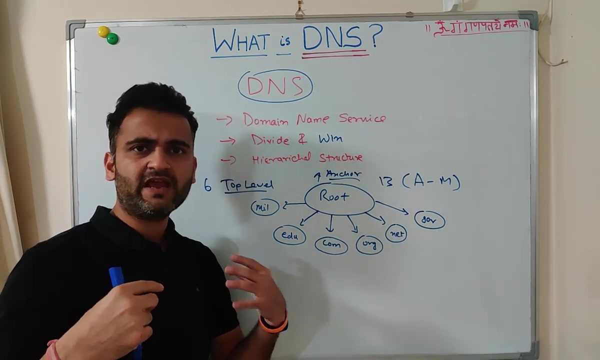 organization. edu is for educational institution organization. dot com is for commercial organizations, any company. that's why you see dot com domain. then there is org, which is non-profit, non-commercial organizations, uses this particular domain. dot net is for your network providers and gov is for government institutions. so now let's take an example to understand. suppose itk funday, my 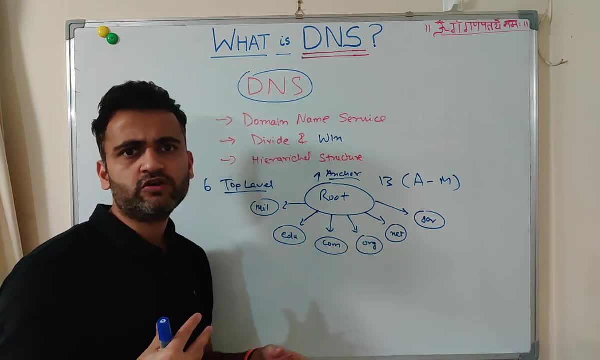 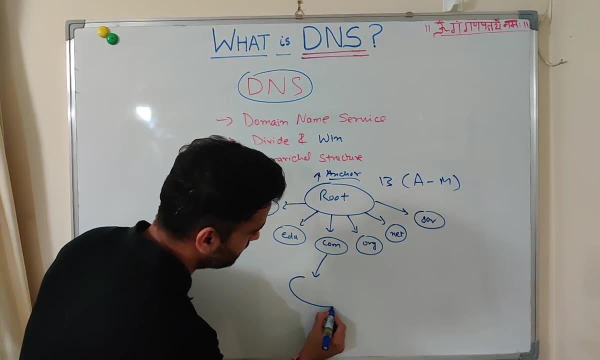 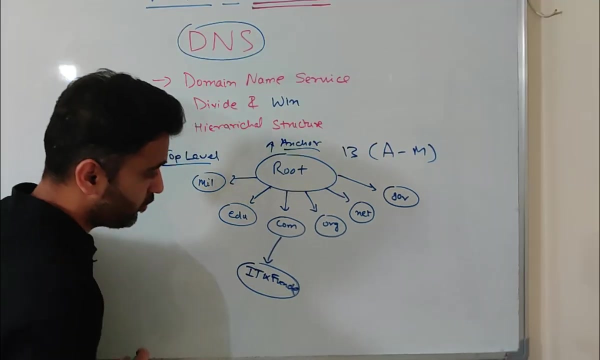 youtube channel. i want to have my own small company to be opened up and i need a domain for that. so pretty much maybe what i can do is i can take a domain here under i, under dot com, and it can be called itk funday, okay, and under this particular domain i can have my office setup okay and my 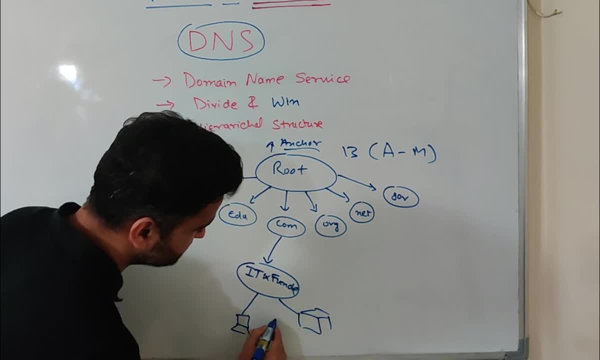 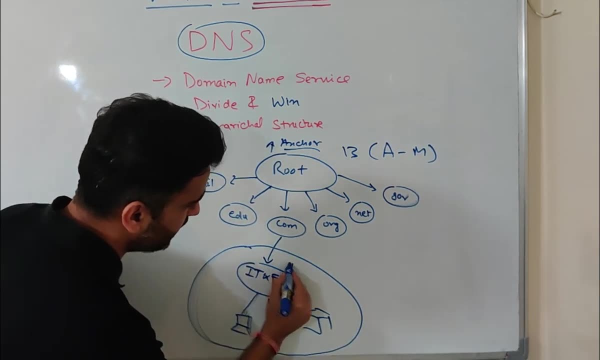 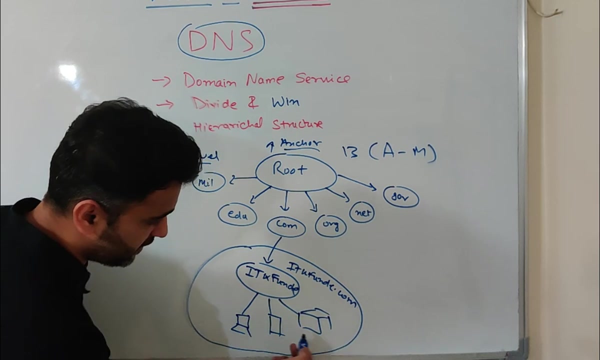 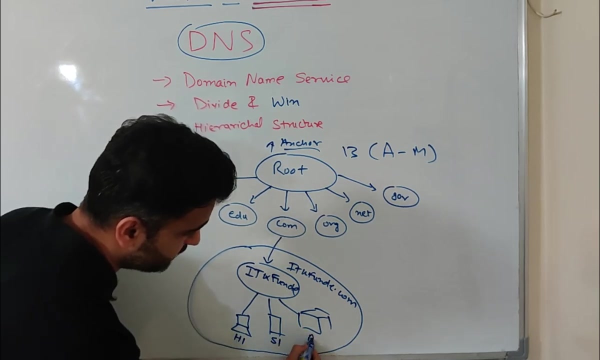 office can have, uh, the, you know, some printers, uh, one may be a server and something like that. so this particular domain will be called as itk funday dot com and then these are the host, uh host devices which are there, so it can be h1, s1 for my server and p1 for my printer. so so what would be the? 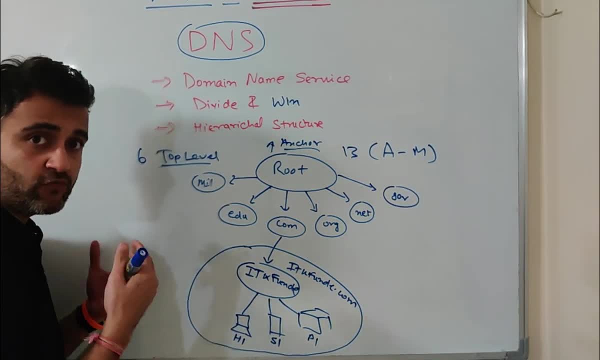 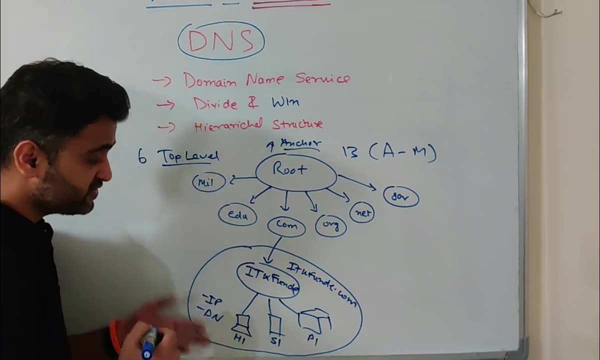 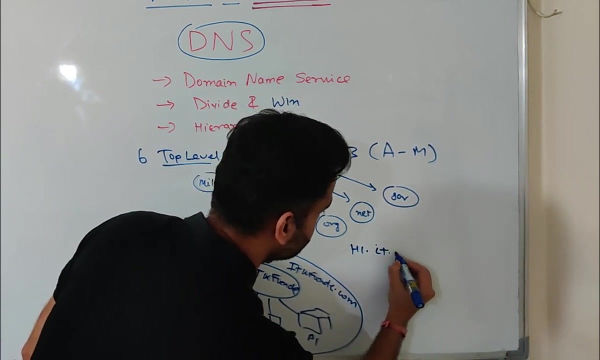 domain name which will be assigned to this particular host. if someone wants to reach it, either it has to know its ip address, which is very difficult, i told you, else it has to know its domain name. so its domain name would be h1 dot it, k, funday dot com, and again a. 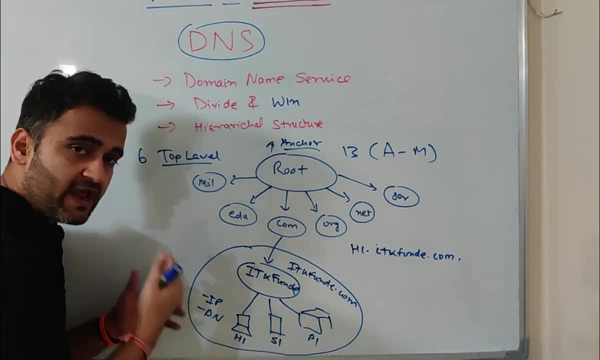 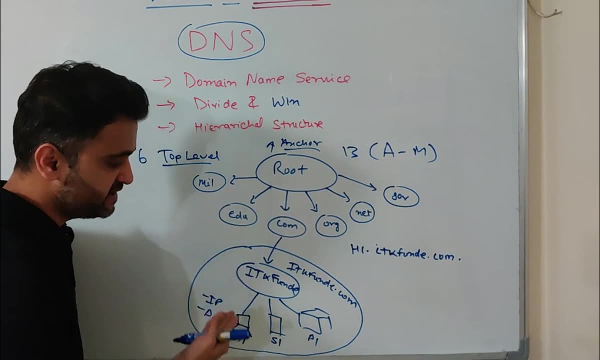 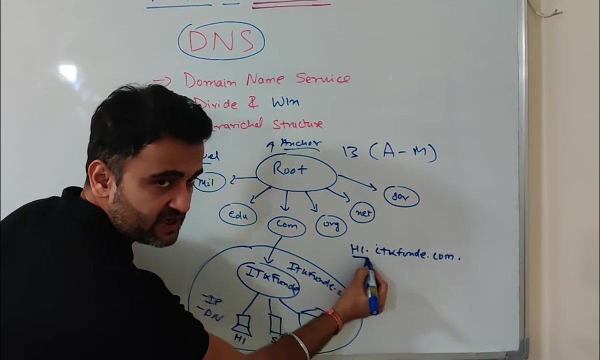 dot. so always understand that whenever you are- uh, you know you are- deriving a domain name, it always follows bottom-up approach. so the bottom-up approach means you will start by the lowest level or lowest level node and you will go go up till the root. so we started with the host. 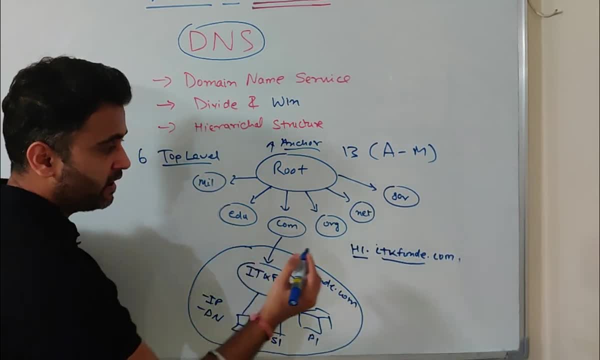 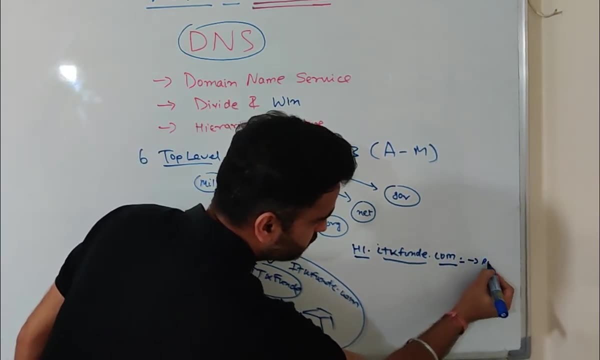 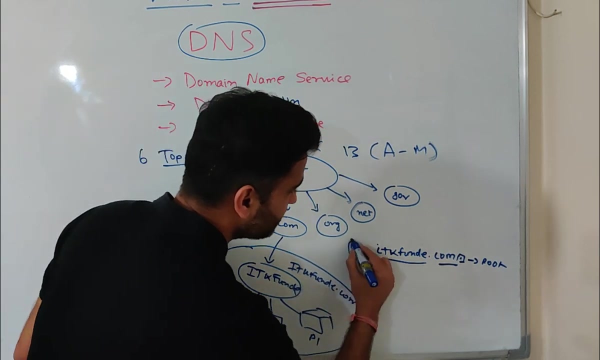 name. then we went to the local domain, which is itk funded. then we went to the dot com top level domain and eventually there is a dot which is your root. but you must be wondering: we never use a dot. well, you don't have to, but this is what is called as a fully qualified domain name. 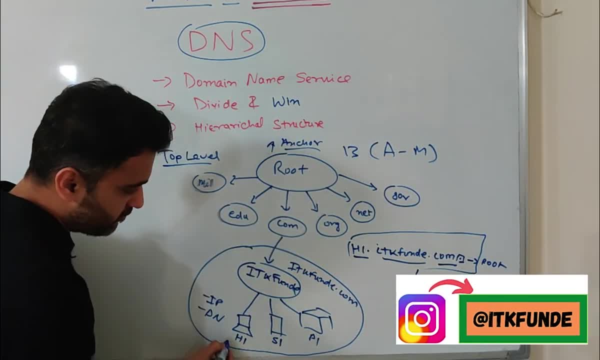 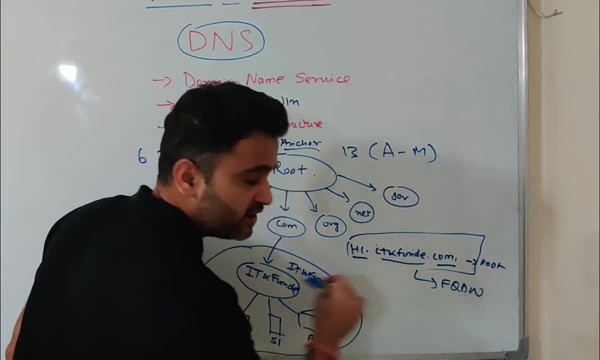 fqdn, Because in this you are traversing right from your lowest level of node up till the root. But if you, in general practice, even if you don't use this, even if you don't use this dot, at the end it will still work. 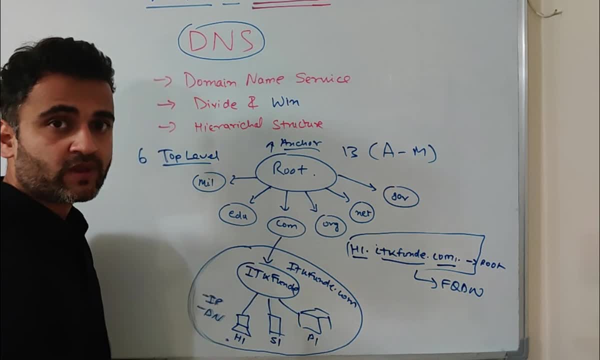 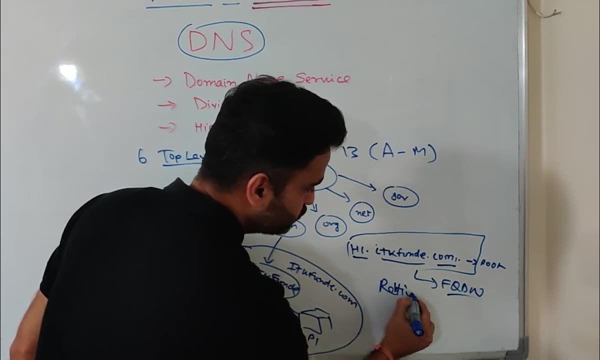 But if you want to test it out, you can put a dot and it will still work. So generally most of the times we don't use FKDN, we use relative names. We use relative names because in relative names also, you know, the DNS is able to identify. 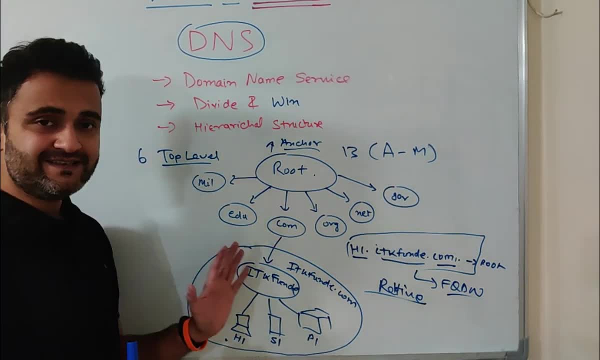 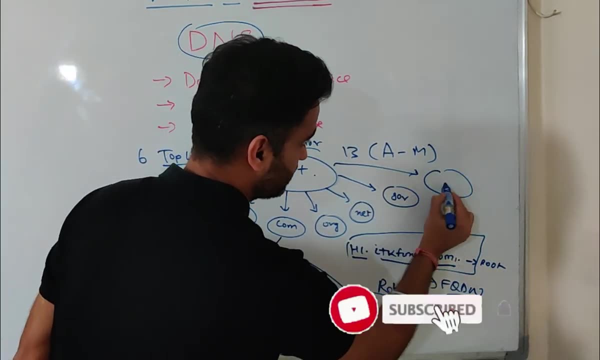 where exactly you want to reach. So this is the structure, But apart from that also, there is a separate domain which is connected with the root, which is geographic domain. So in geographic domain, what happens is that different countries have dedicated domains. 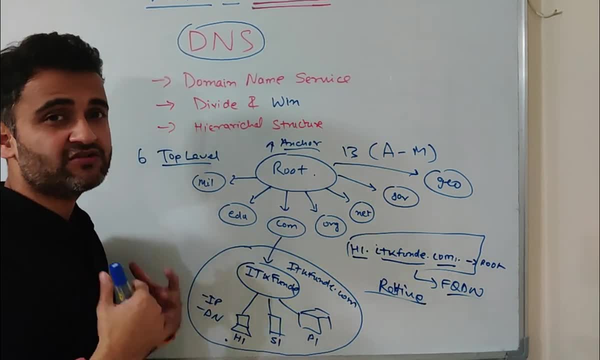 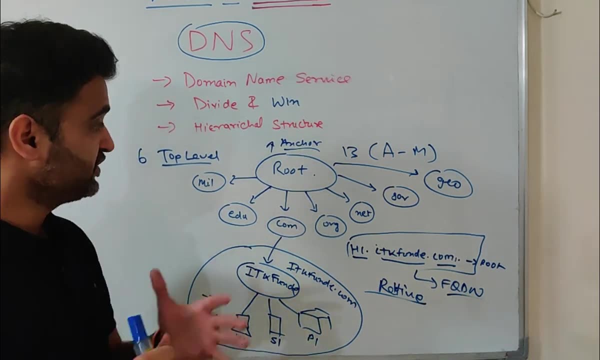 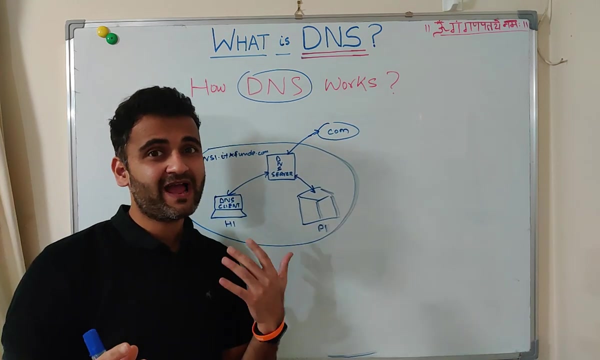 like India has dot in, UK has dot UK, US has dot US. So even in those areas, in terms of geography also, the domain name has been distributed. Friends, now let's understand how DNS works, How DNS exactly works. But before that let's go 10,, 15 years back, when we used to have a mini DNS in every computer. 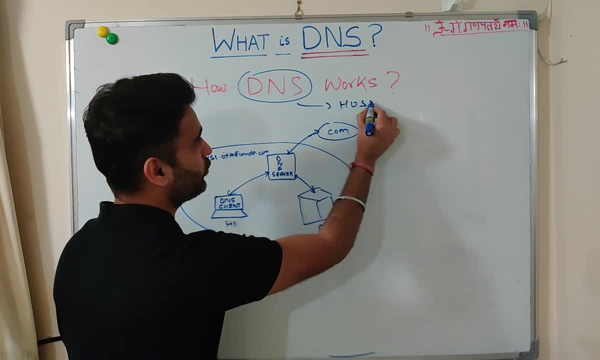 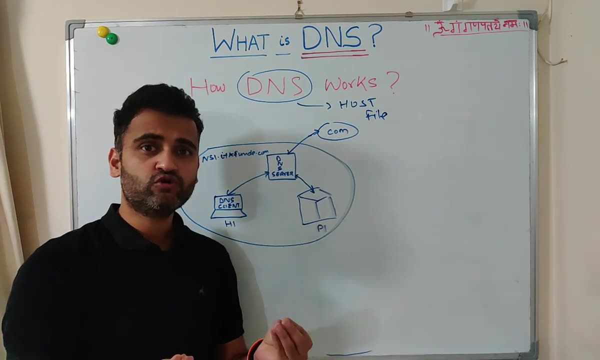 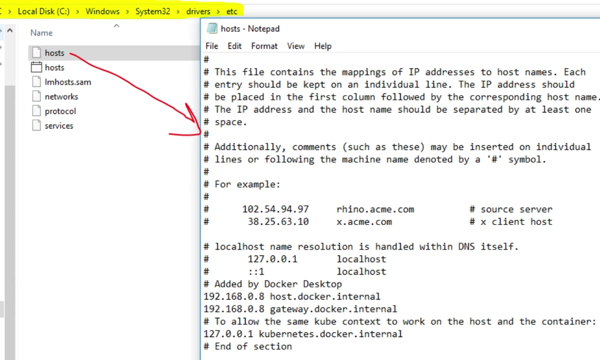 which used to be called as our host file. You remember this. Maybe you might have used it, might haven't used it. In Windows you used to have, and still today you have host files in which you maintain the IP address domain name you can maintain. now it is not feasible because the network 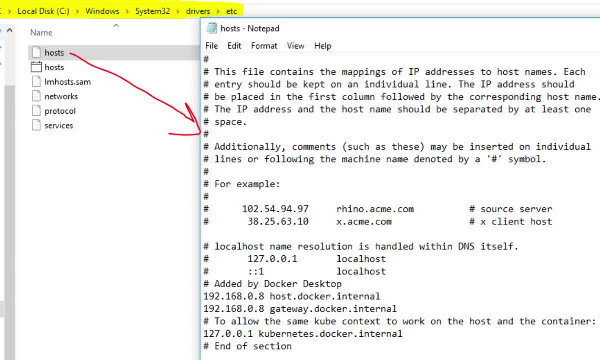 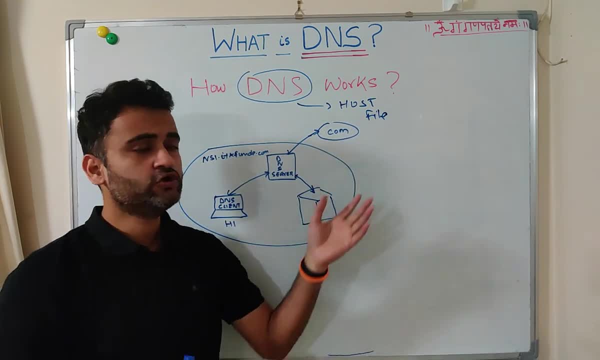 has grown that much, But in earlier days the network used to be very small So you used to maintain that host file. wherever you want to reach a device over the network, You used to go to that host file. check the domain name and the IP address. 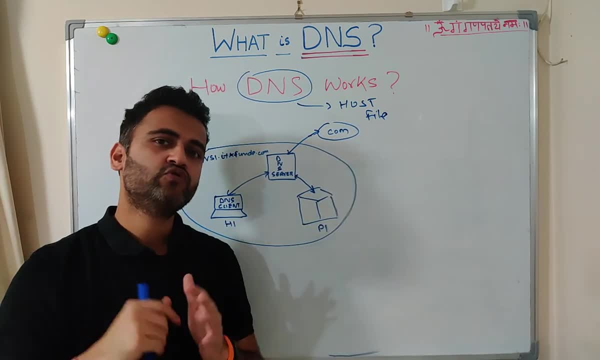 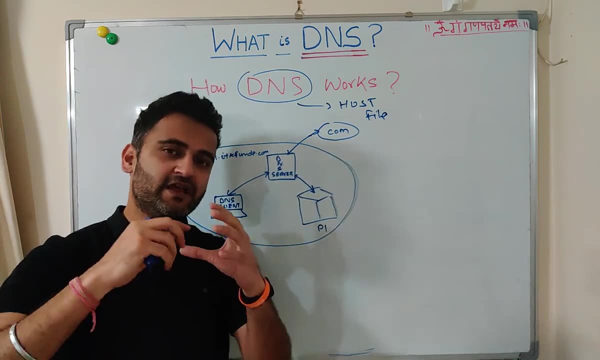 Everything is there in that particular host file And from there you used to traverse to that particular destination. But now host files are no longer in use. But you can imagine that if you understand the functionality, pretty much the same functionality is done by us. By our DNS servers Till today. if you put something in the host file, then by default Windows checks first your host file and then only it goes to the DNS server, because it is so quick. you do not identify the difference, But you can check it. 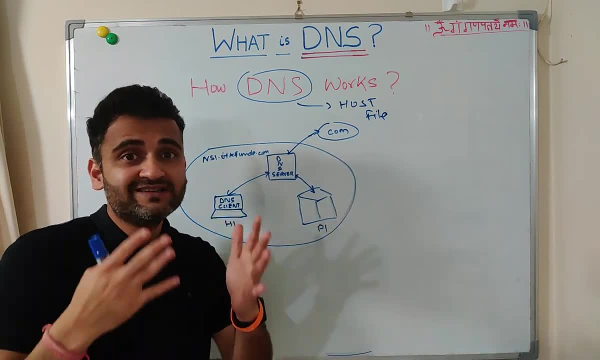 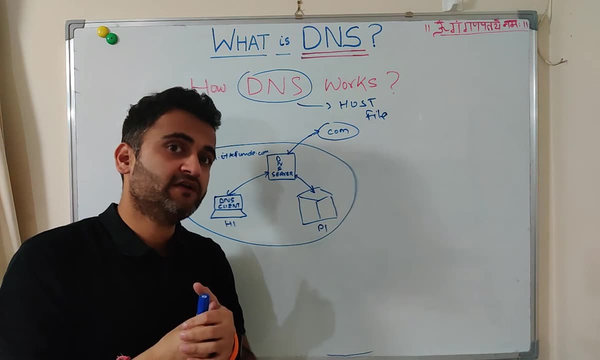 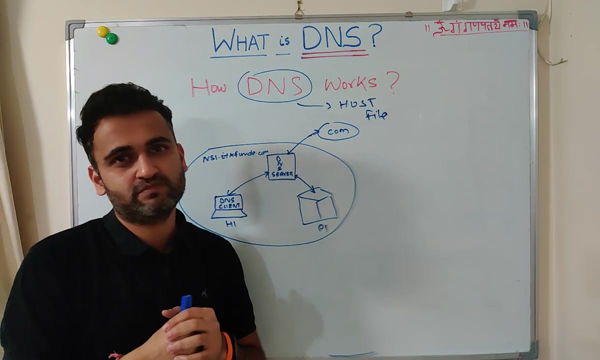 You can put something. So sometimes during performance troubleshooting this step is used, wherein you try to put something in the host file and see whether it has any difference in the overall performance Sometimes. But now it is no more used that much because the network has become so so scalable and 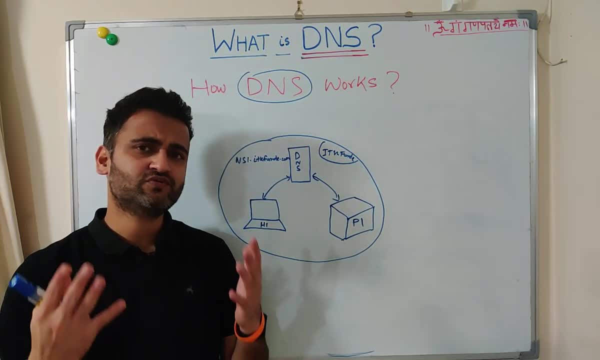 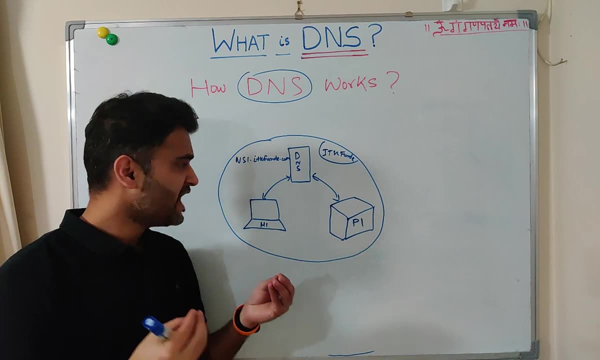 so fast Moving on, Let's understand how exactly DNS works. So every machine which is trying to connect or trying to connect to the Internet, for example, is actually having a DNS client in it installed, And then what it does is that suppose it has to reach to a particular device over the network. 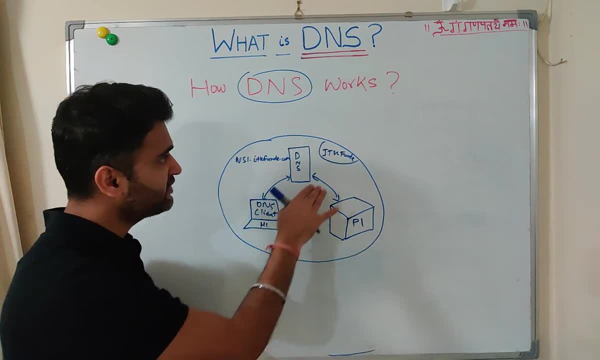 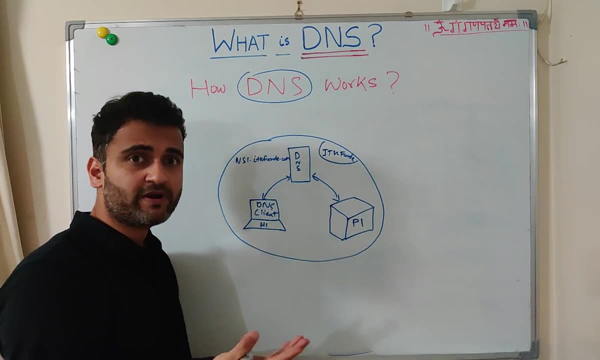 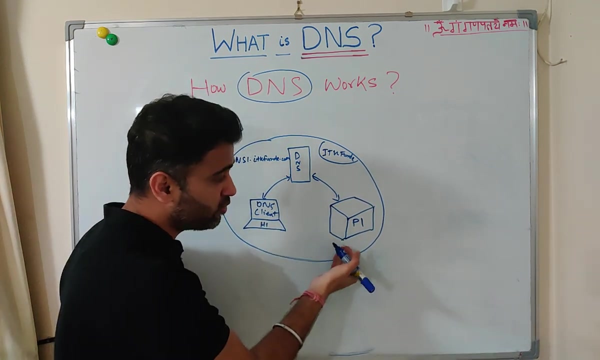 In this case my particular host in my particular itkfundedcom domain. I have my computer and I have a printer. So my computer wants to connect to my printer to give a printout. So it is in the same local domain. So it is h1.itkfundedcom. 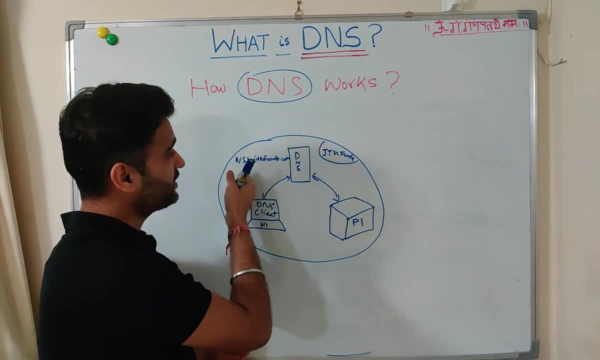 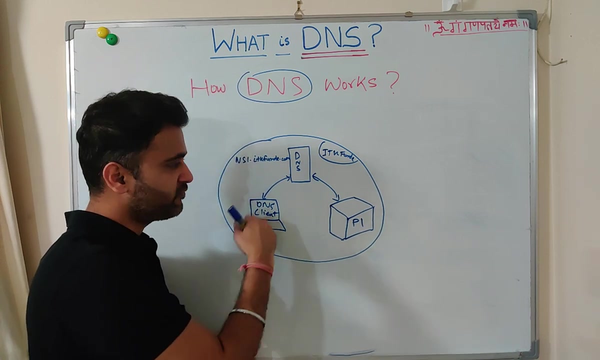 This is p1.itkfundedcom And I have also hosted like a DNS server to resolve these queries, Obviously because I'm maintaining my own domain and a DNS server, a name server, which will resolve this for me. So my host will run a DNS query. 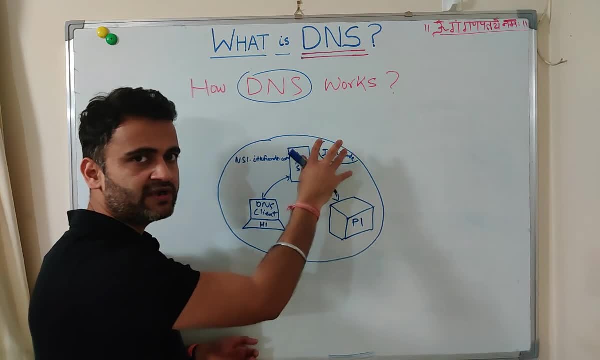 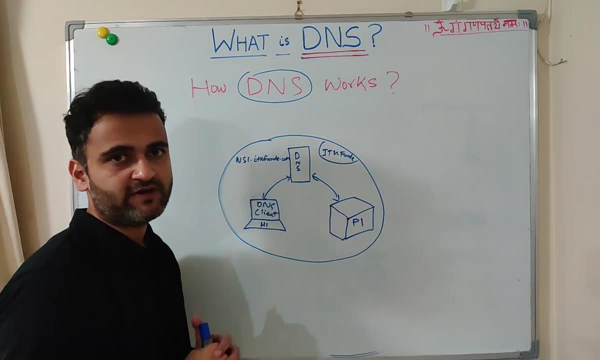 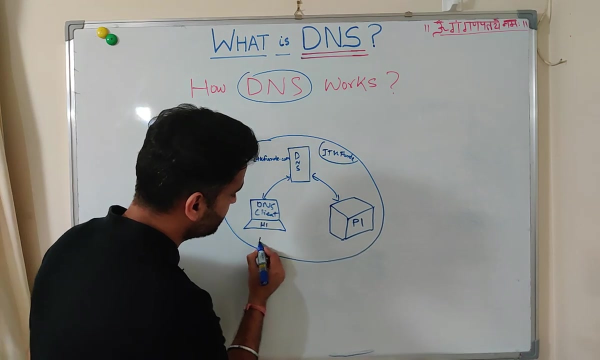 If it wants to give a printout, it will run a DNS query, My local DNS server will respond back with the IP address of this printer and then it will be done. So it will be very, very straightforward. But what if my computer wants to visit a website which is wwwwikipediaorg? 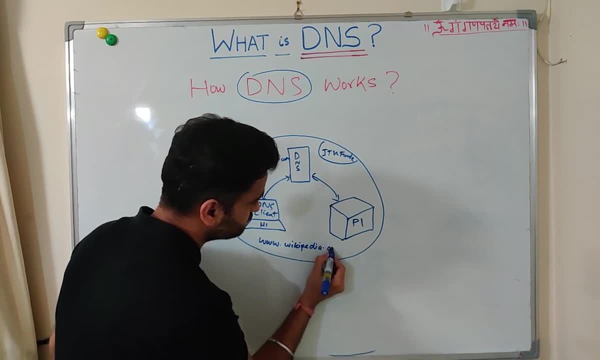 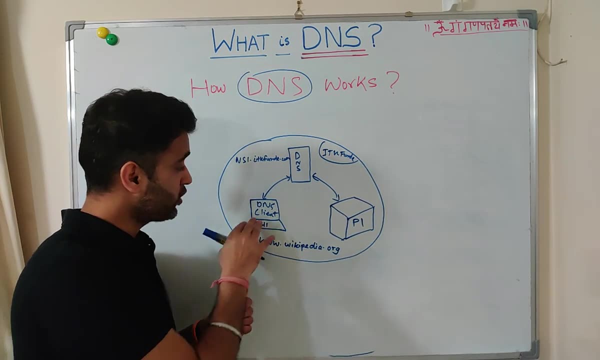 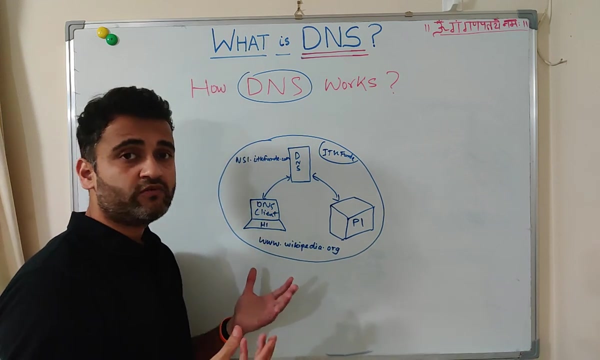 Okay, Okay, Now this particular website, when this will be entered on my laptop, maybe, or this particular host on the browser. my DNS server won't have a clue that exactly where this has come from, because it has never seen this address. 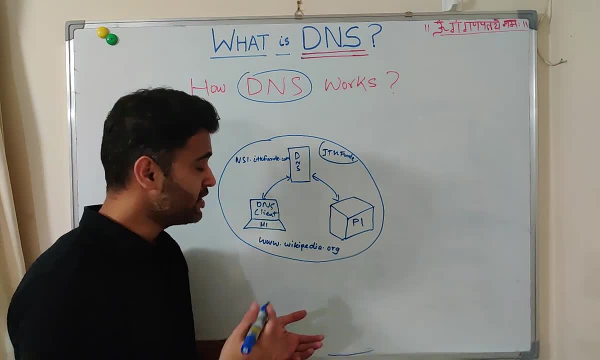 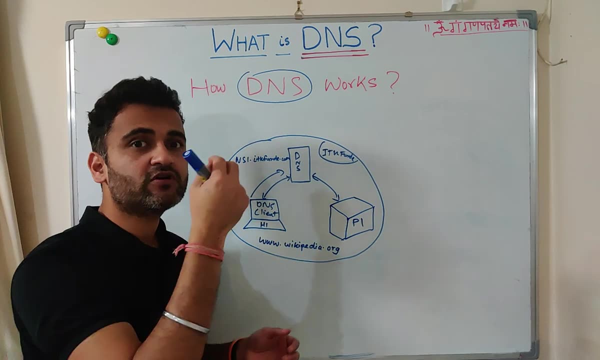 It is nowhere in its address book. So in that case, the DNS query. So one more very important concept: whenever you are querying anything to the DNS server asking for some address, IP address, Then it is called as a DNS query. 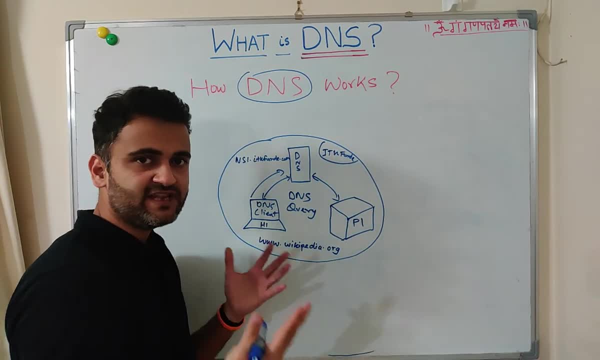 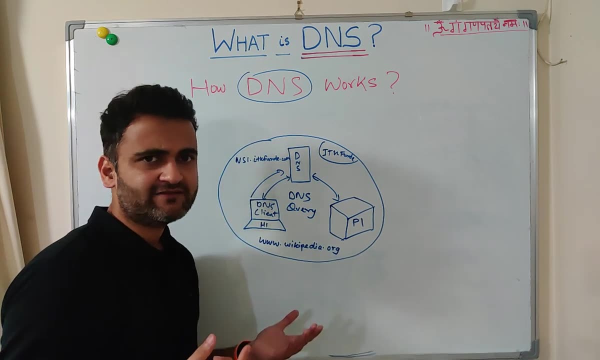 Okay, So you will fire a DNS query. Obviously, it will not have a reply. It will not have an answer to your query, So it will respond back saying that I do not have this, but maybe my parent, so my parent. 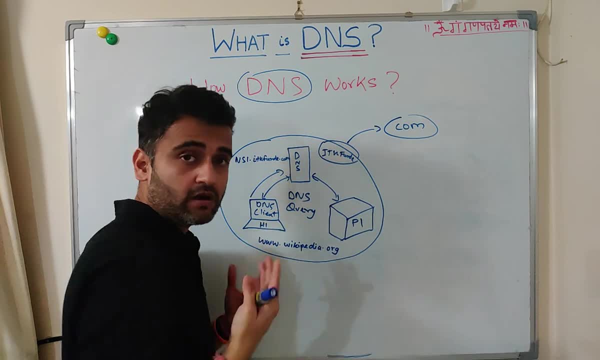 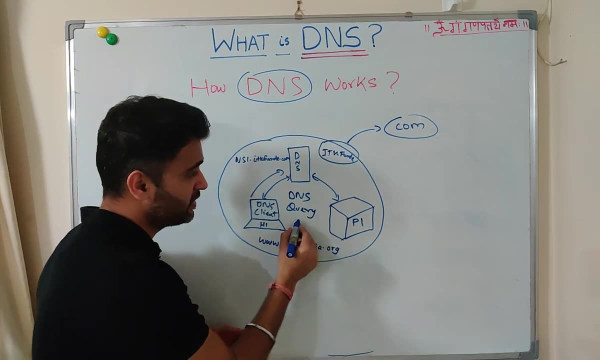 which is the com domain, might have an answer to this particular query. So now, even the DNS queries are of two main types: The first one is the domain and the second one is the domain. So the domain is the domain, The domain is the domain. 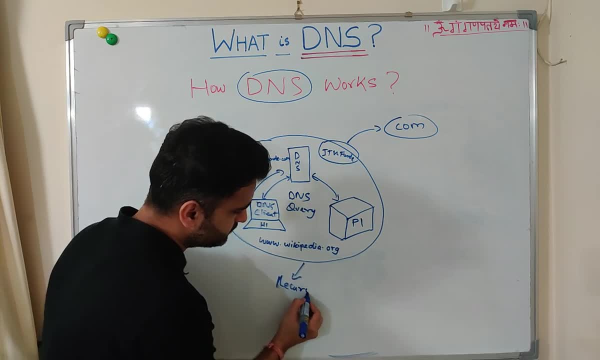 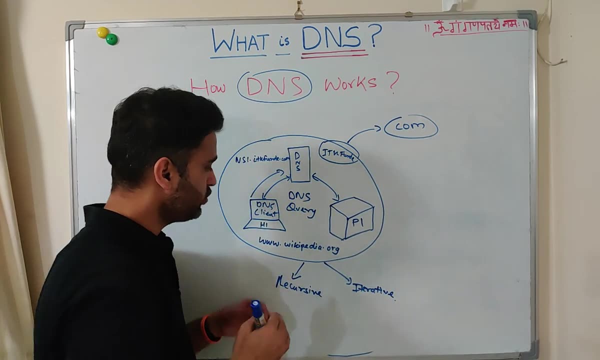 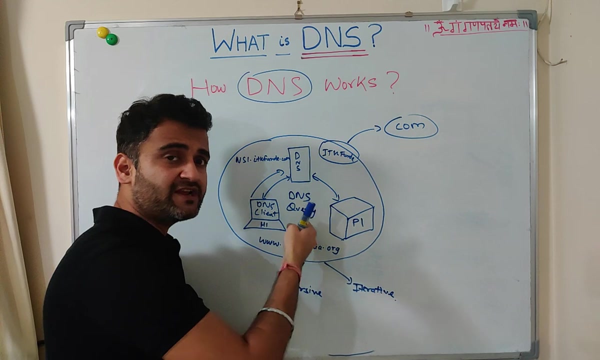 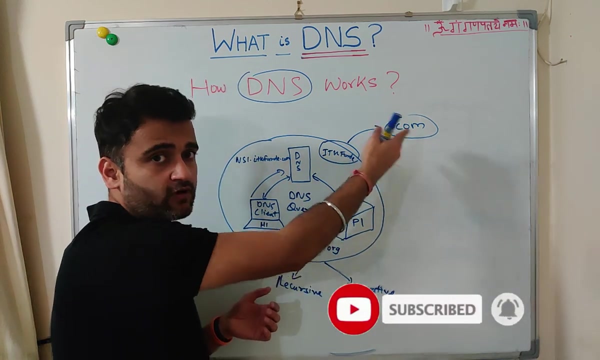 what are those types? one is recursive and second is iterative. so in a recursive query, whenever a dns client queries to a dns server, that particular dns server is obliged to either respond back with the ip address or tell that okay, i can't find it, but maybe you can look for this in the uh in the other domain. 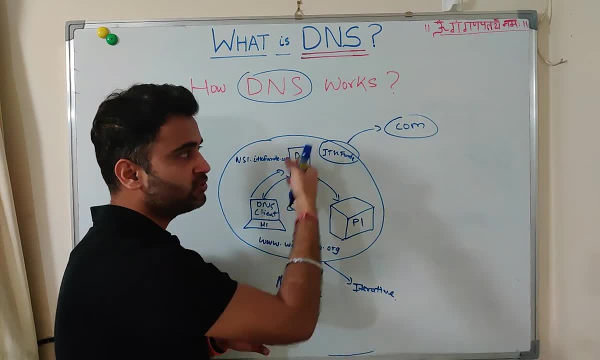 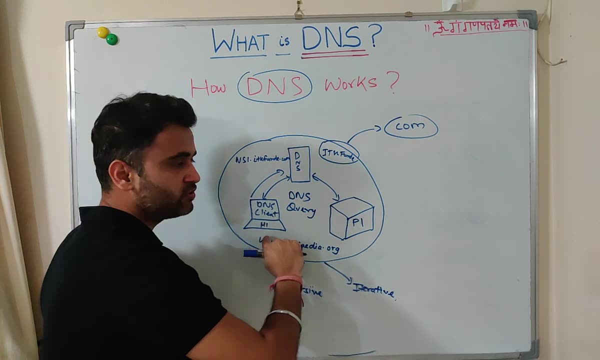 available, so it will pass on that address and then this particular client can connect directly to the dot com domain. but generally it is a mix bag. so firstly, suppose my computer talks to this particular dns server, so it will send a recursive query. okay, so this recursive query will be here. 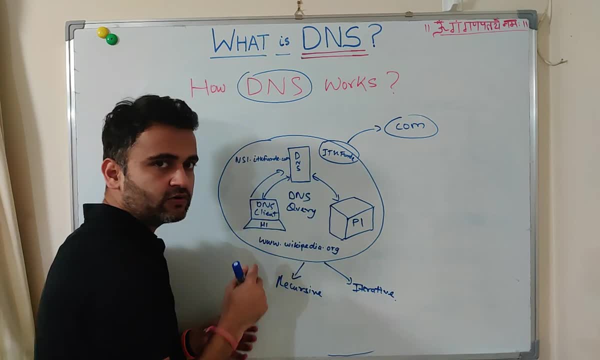 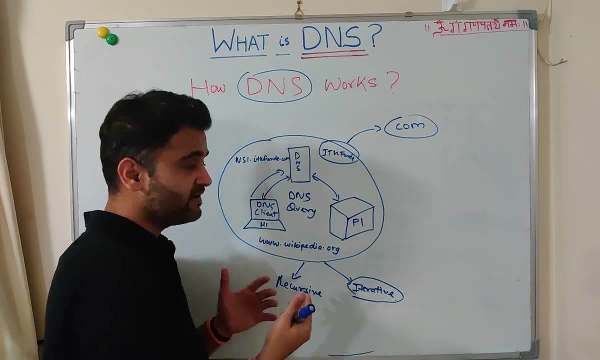 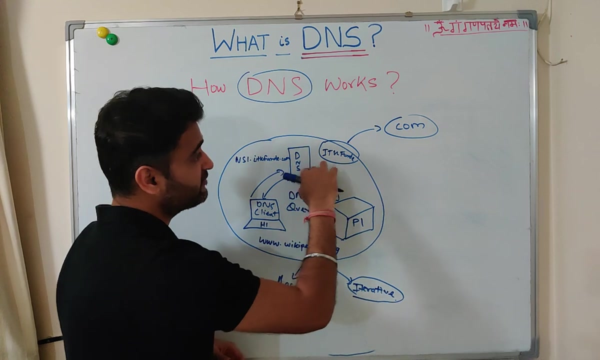 go on to this particular dns server. my dns server will reply that okay, i do not have it, and then it will fire an iterative query. now, what is iterative? iterative query is something where it the dns server, takes the load of finding it out for you. so what it will done, what it will do is it will fire an iterative. 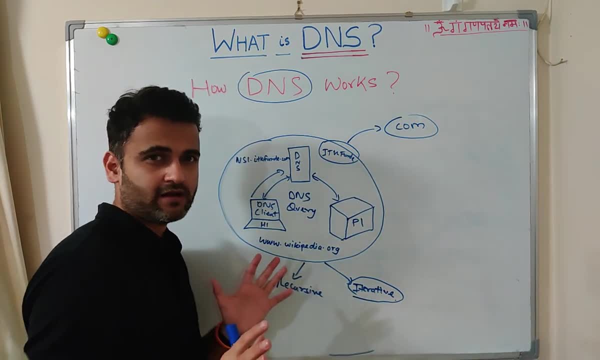 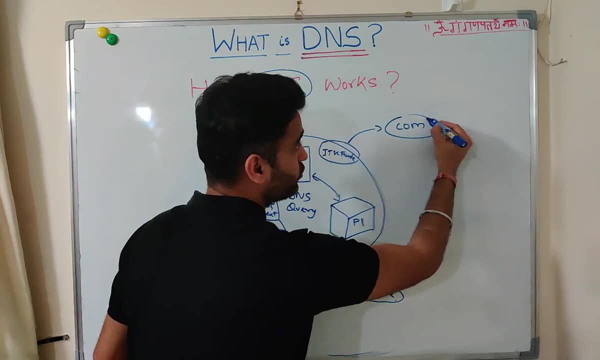 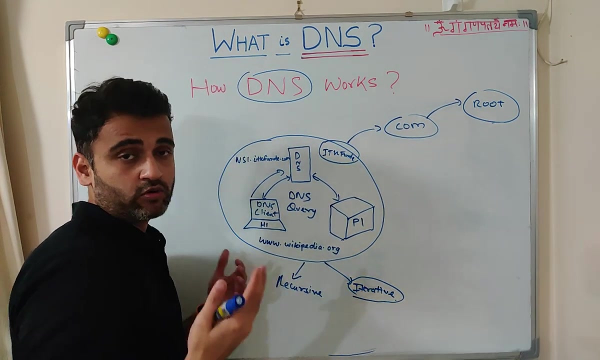 query to the dot com domain, asking that: do you know anything like wikipediaorg on which the dot com domain can again fire an iterative query to the root domain? because even the dot com domain does not have a clue about what is this? wikipediaorg now, root being the parent, the master of all will say that okay, let me find among all my top level domains. 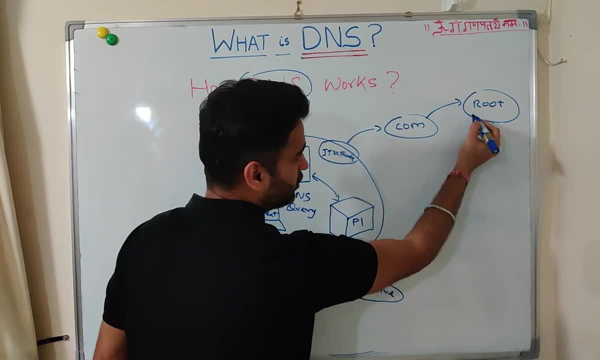 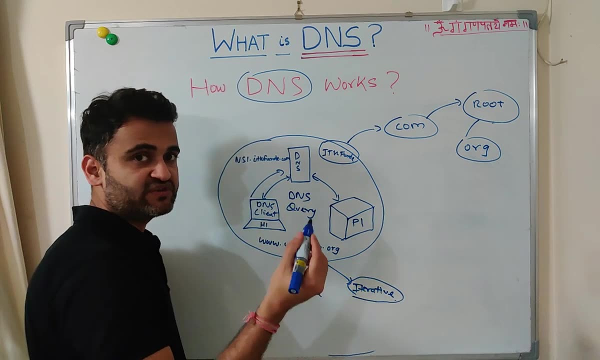 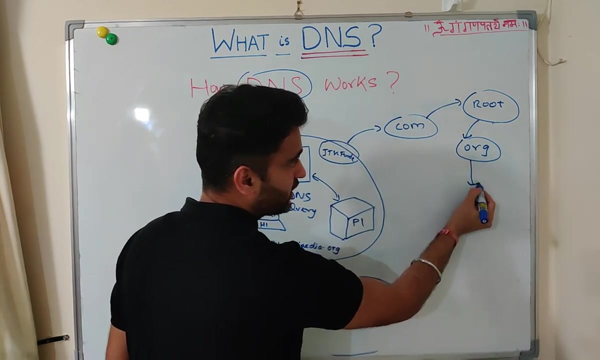 i can find this particular child. so it will query all the different domains and then it will find out that dot org has something, some chances of finding this particular wikipediaorg. so it will. it will pass on that query to dot org. dot org will again find out among its multiple children's and 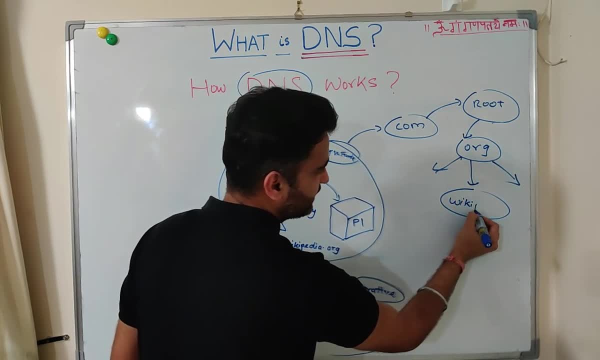 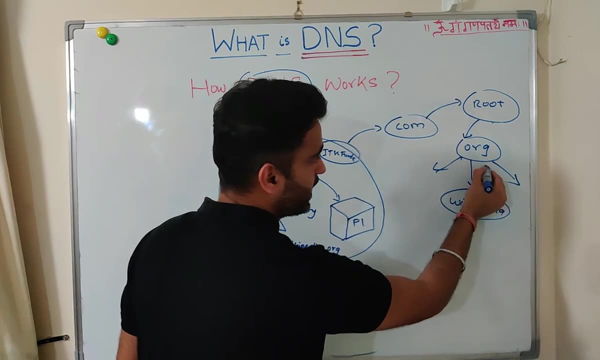 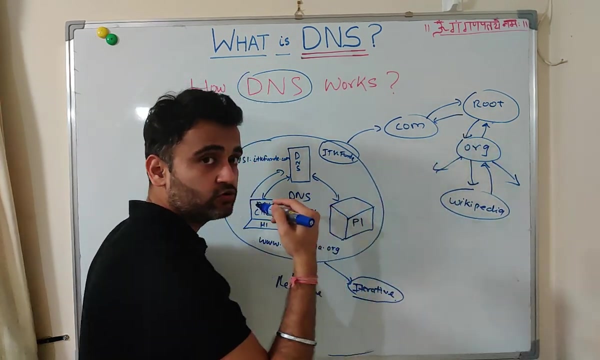 it will find that, yes, there is a wikipedia child sitting here which can serve this particular query. so this particular wikipedia domain will respond back to dot org with the ip address of the server. again, dot org will respond back to the root. root will come back to the dot com domain. dot com will send back to my domain, which is itk. 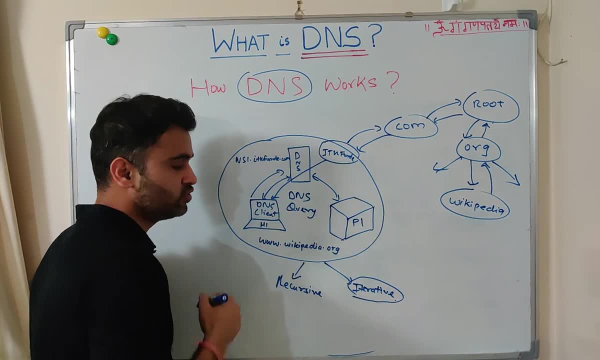 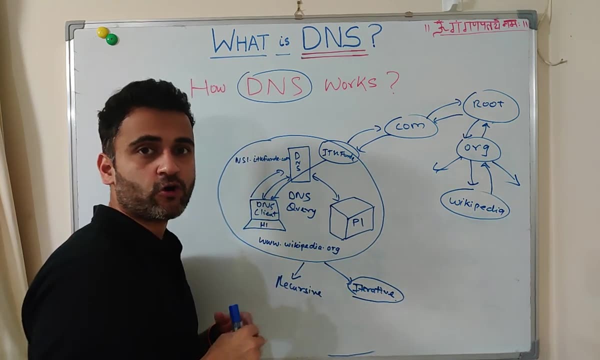 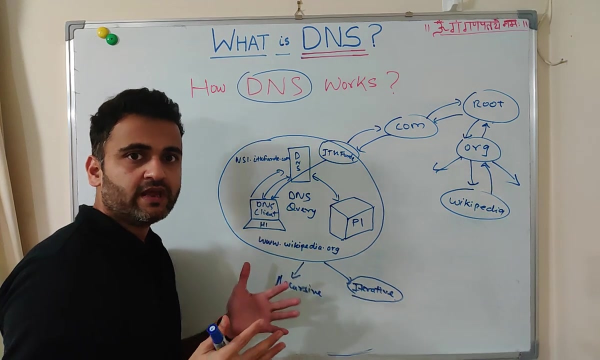 funday, and then i will send it back to my client machine which is having, uh, you know, the dns client, which is actually waiting for this wikipediaorg. now, when i say all this, it looks like a very, very lengthy process, but in network it happens in a, in a, you know, in a fraction of a second. so it is very, very quick. you don't even 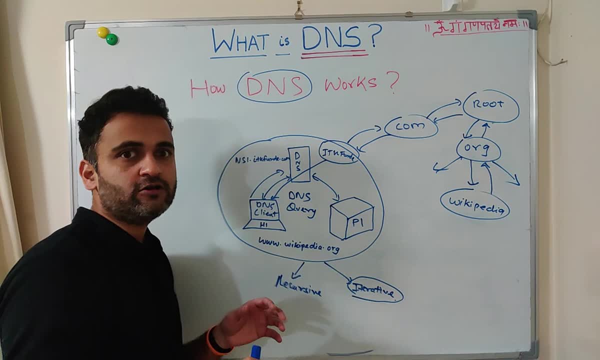 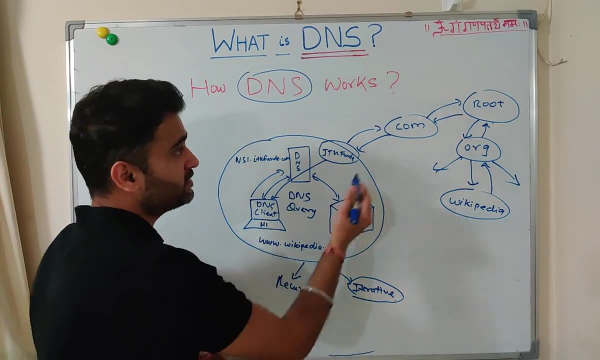 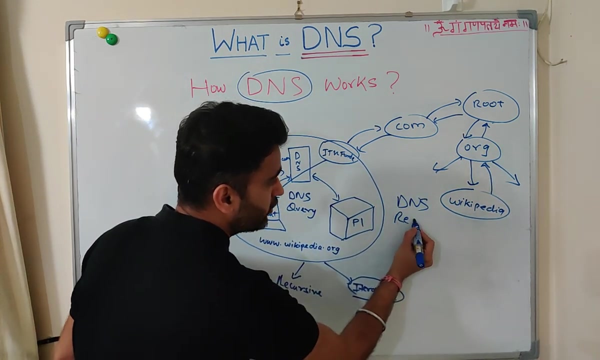 realize when you did all that as soon as you hit enter you feel that everything has happened very quickly. but behind the scenes so much happens. but there is an important concept again that once this whole process has completed, which is called as dns resolution, so as the name suggests, we are trying to resolve the dns query to an ip address. so this process is 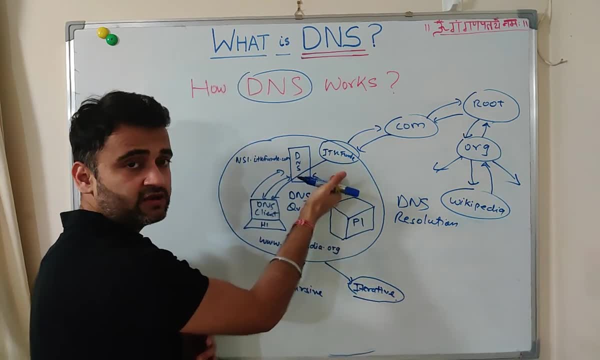 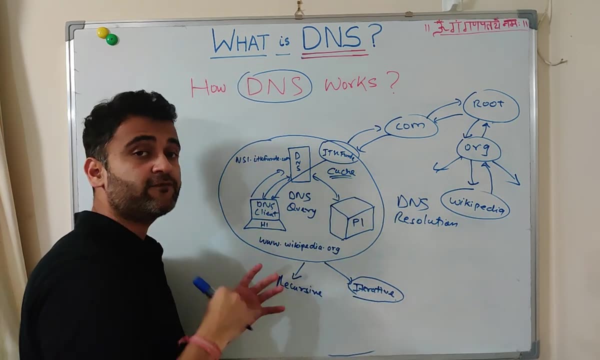 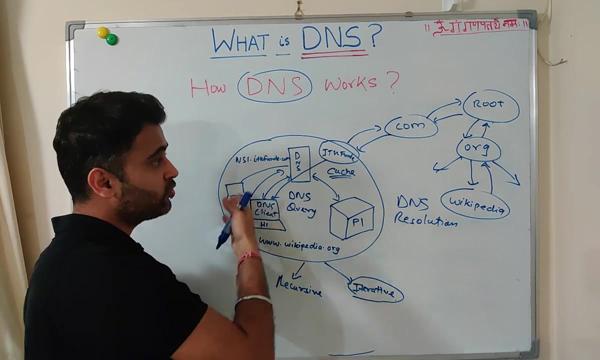 called as dns resolution. once my domain, my local domain server, gets the ip address of wikipediaorg, it will cache it, it will store it in the local cache for future use. so suppose another computer, suppose another computer is joined in my network, it also wants to go to wikipedia. then this whole. 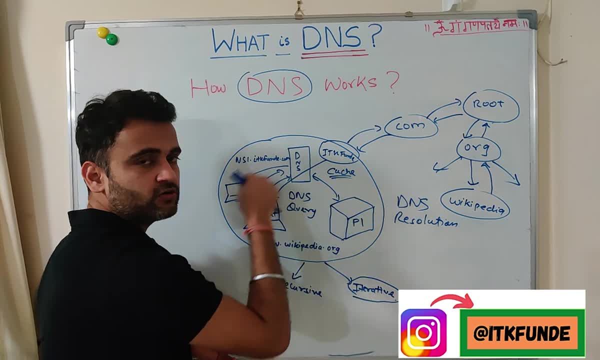 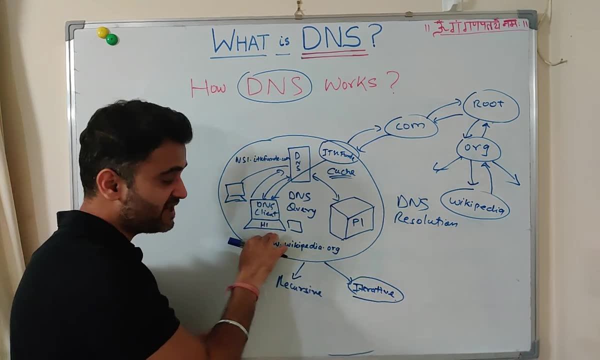 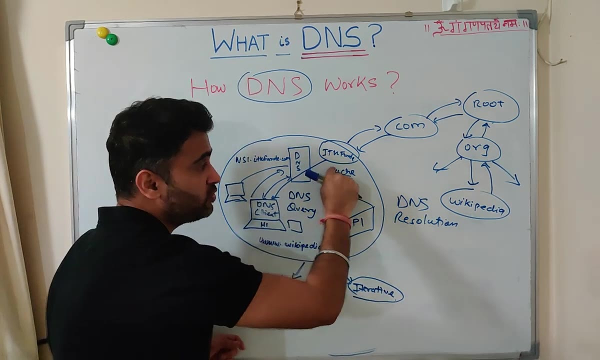 cycle won't be required. my uh, my local domain, will pass it on that ip address to my new uh computer. so at the host name, at the host level also, there is a caching which can be done so that next time the computer does not even have to go to the local domain, it can directly go. 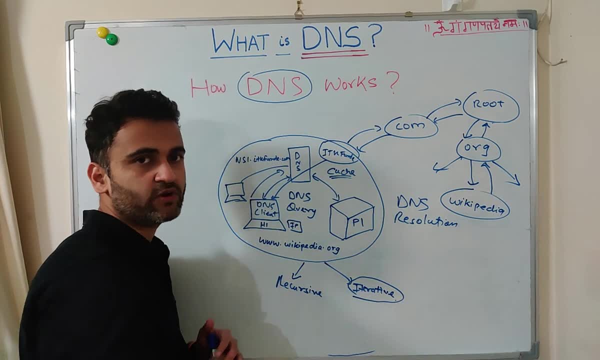 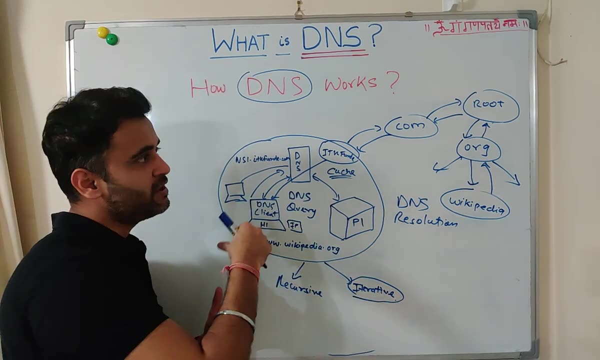 with the ip address which it has- uh, you know, which it has got from the previous query. so this is the whole concept, on top of which this whole dns works on. as you can understand, all this happens so quickly that you don't even realize. but this is very, very important concept, guys, because 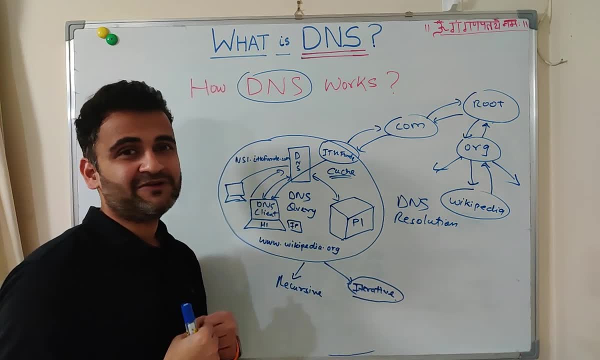 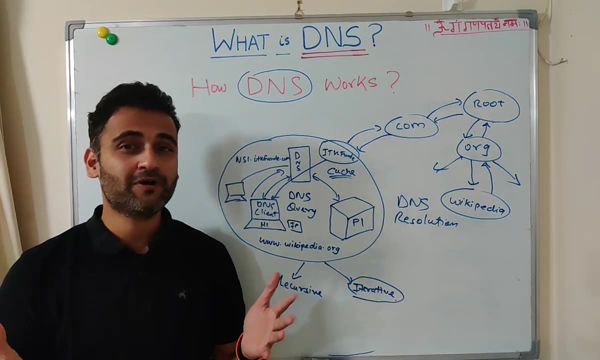 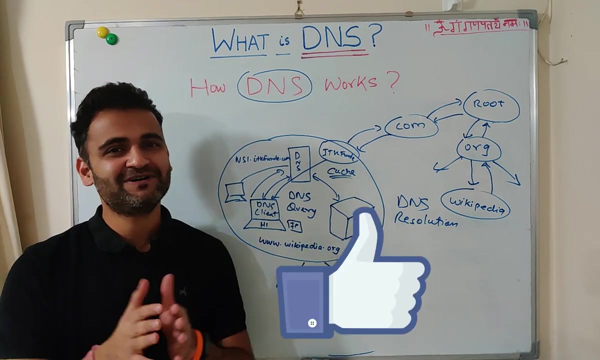 without this, i think the whole internet, the whole world, will die, would not be able to connect to itself using the power of networking. I hope you now know a bit more about DNS and how important it is in the field of networking. so if you found this content useful, by any means, please hit the like. 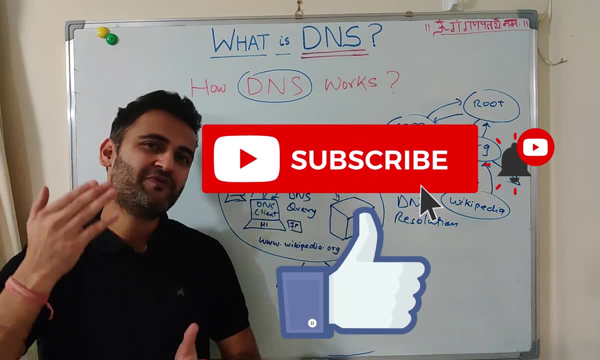 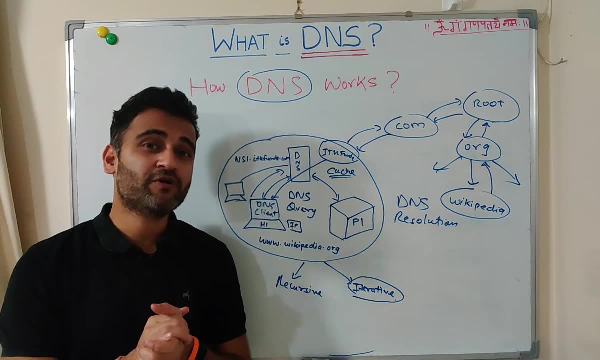 button. hit the subscribe button and the bell icon so you exactly know when I upload my next video. and yes, let me know in the comment section what you would want to learn next. I am getting a lot of requests to make videos in the field of data, like data engineering and data pipeline, so definitely, we will be doing.